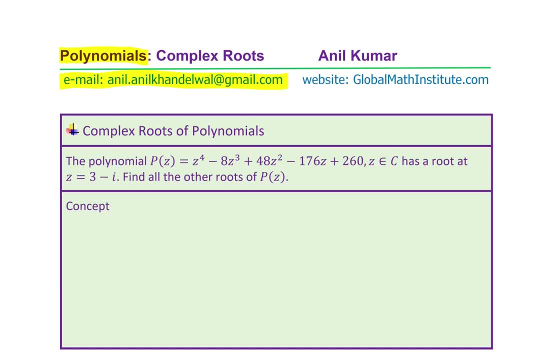 on the address given In previous days, I've got a few inquiries about how do we find the complex roots of a polynomial. Based on the questions received, here is one, an example, which will help you understand solution of questions regarding the same. So we'll discuss. 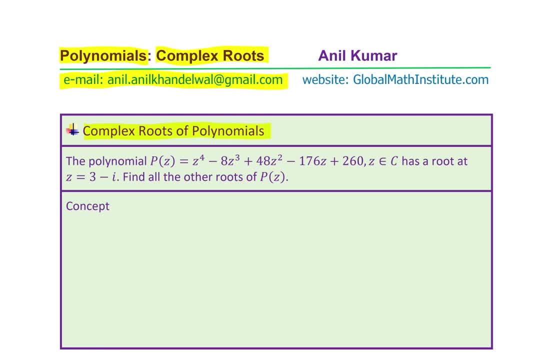 how do we find complex roots of a polynomial? in this particular video Question here is the polynomial P of Z. So when we write Z it is supposed to be a complex number. So Z to the power of 4 minus 8Z cube plus 48Z square minus 176Z plus 260, where Z belongs. 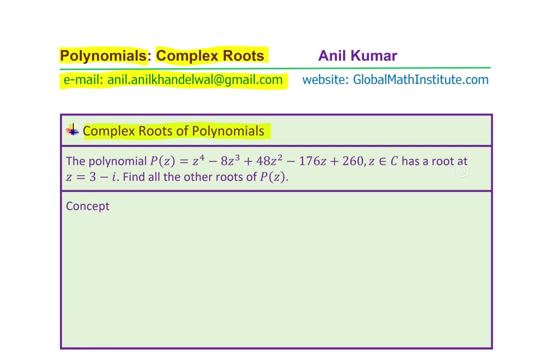 to set of complex numbers has a root at Z equals to 3 minus. I Find all other roots of the polynomial PZ. So when I say I, it really means what? So so I means it's equal to square root of minus 1, right, That's. 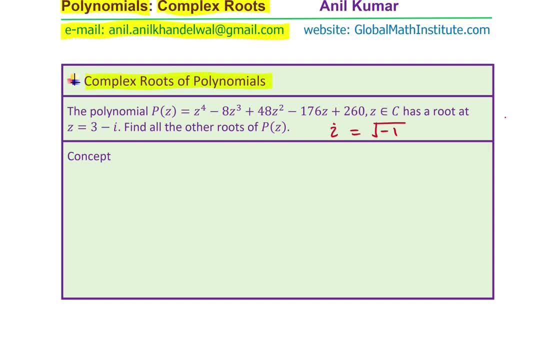 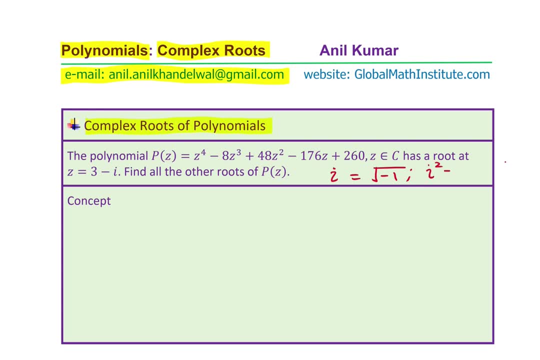 the set of complex number. Or you can also say: or you can also say that I square is equal to minus 1, okay, So that is how it is. I'd like you to pause the video, answer this question And then look into my suggestions. Let me begin with the basic concept. So we are saying that? 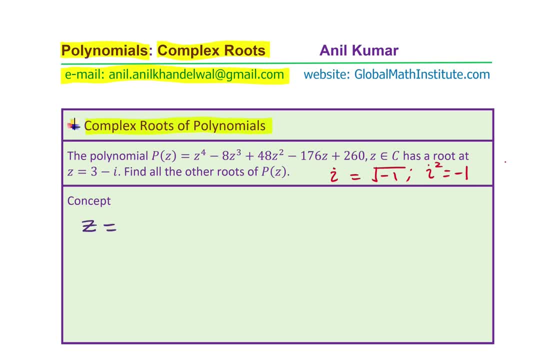 one of the root is at Z equals to 3 minus I correct. As you know, the complex roots are always in conjugate pairs, right? So remember, complex roots are in conjugate pairs. So what does that mean? It means if one root is at three minus I, the other root will be at. 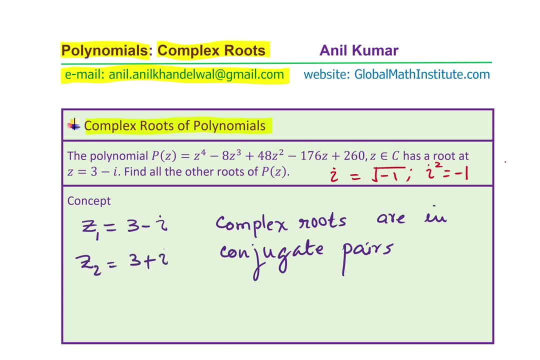 three plus I, the conjugate of thatoun helping toanging dasce Tu Re Correct. Now, once we know that there are these two roots, it means that you'll be able to imipermane this by vector. So root basically means I could write this as Z minus three minus I, as one of the 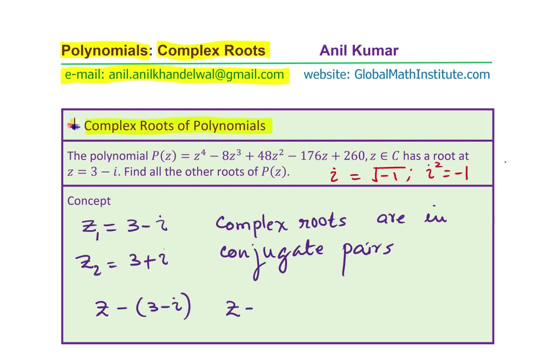 minus i as one of the factors. the other will be z minus 3 plus i, correct. So if I multiply these two factors I'll get my quadratic term correct. You can say quadratic factor, correct. So one of the quadratic factors will be there. 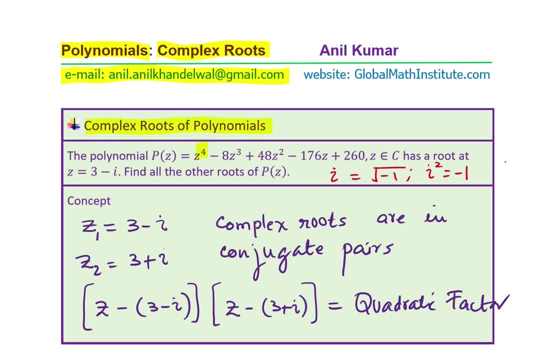 We are working with a quartic equation. do you see degree 4?? So this is a quartic equation. We can say quartic polynomial. So if I divide this by a quadratic factor, in that case the other factor will be a quadratic. 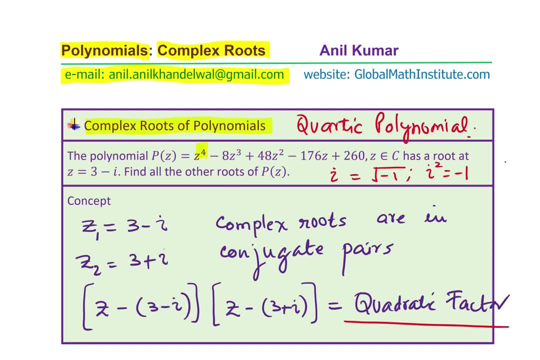 factor, and then we can use the quadratic formula. right, So we'll do division And that will give us the other roots Using quadratic formula. is that clear to you? So the concept is absolutely clear. I'd like you to now pause the video. do the needful. mainly, you now know that there are 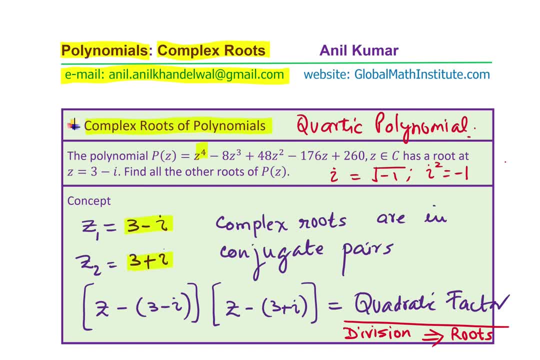 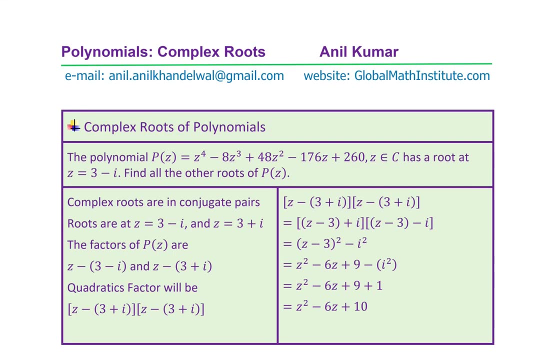 two roots given to you, 3 minus i and 3 plus i. Just multiply these two factors, get a quadratic factor, perform the long division correct And then get the roots. Let's begin. So first thing, first we'll try to find what are the, what is the quadratic factor, and 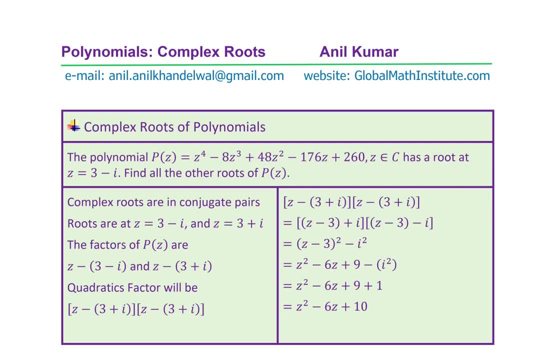 then we'll further go with division. So, as I was saying, the complex roots are in conjugate pairs. So if we know that 3 minus i is one of the roots, in that case the other root is 3 plus i. 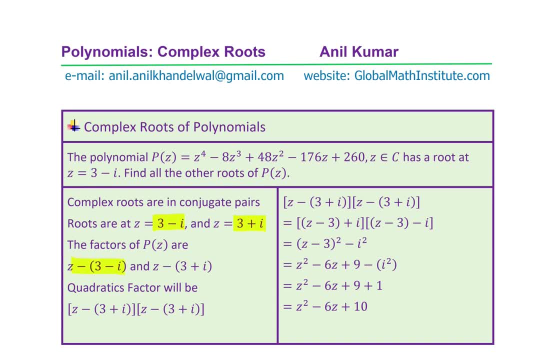 So that means z minus 3 minus i and z minus 3 plus i. z plus i are the two factors. Let's multiply these two factors to get the quadratic factor Perfect. That's the summary of what we discussed. So let's now do the division. 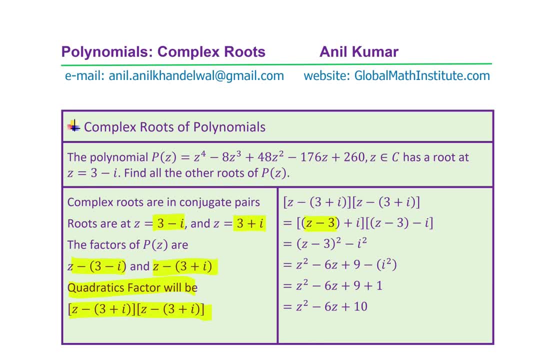 So first step, first open this bracket. So you get z minus 3 plus i and z minus 3 minus i. Now it becomes very simple to multiply, right? You know what is a square minus b square equals to right. 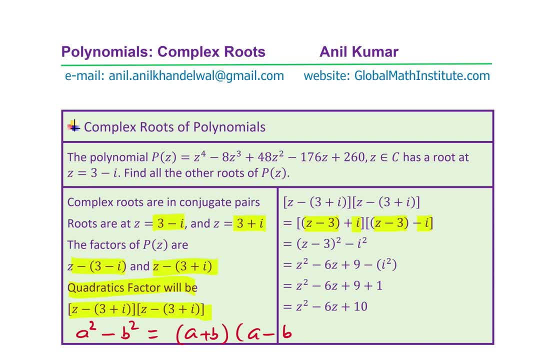 It is a plus b, times z minus 3.. Times a minus b, And we have used this property here, and so we got a which is z minus 3 and b which is i. So we get z minus 3, whole square minus i square. 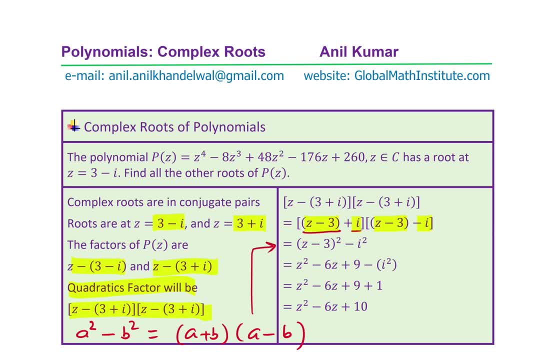 Now expand this expanding using the formula, as you know, a plus b. rather I may write a minus b, since we have minus. in this case, whole square is equals to what a square minus 2ab plus b square, Right. 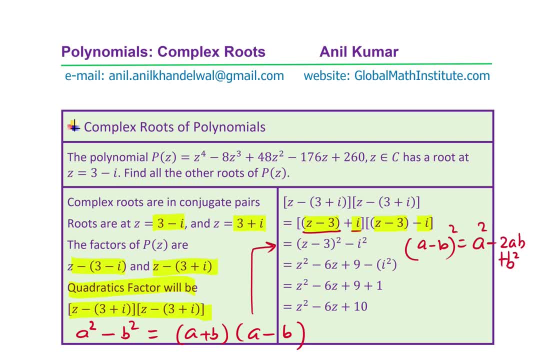 And that's what we did. So a square is z square minus 2ab gives me 6z minus plus 9.. And what is i square? Well, i square is minus 1 and therefore minus, and minus becomes plus 1.. 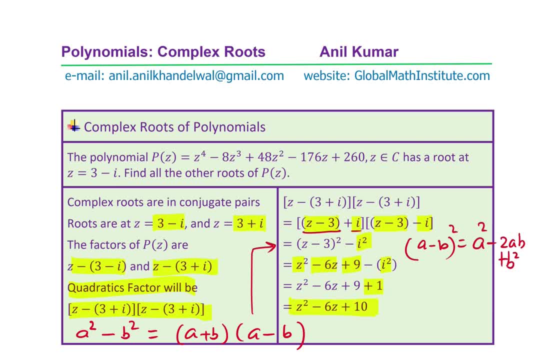 Adding 1 to 9, we get 10, and we do have the other quadratic factor, which is z square minus 6z plus 10.. Right Where z is a complex, Right Where z is a number. Is this clear to you? 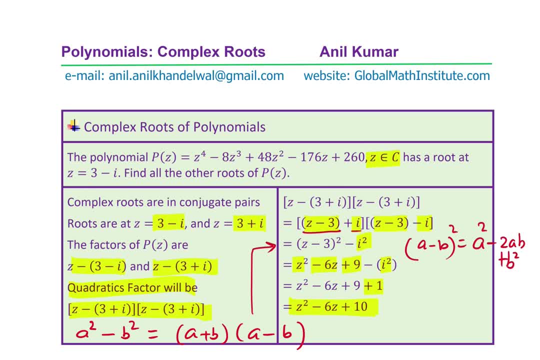 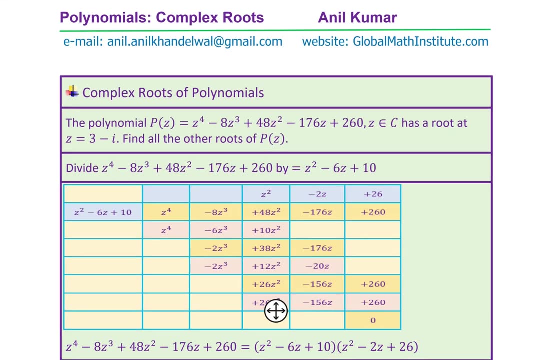 Have a good look at it. Try to understand how did we find the quadratic factor using the two roots, and these two complex roots at 3 minus i and 3 plus i? Correct, Now we need to perform division. Let's perform long division to find the other factor right. 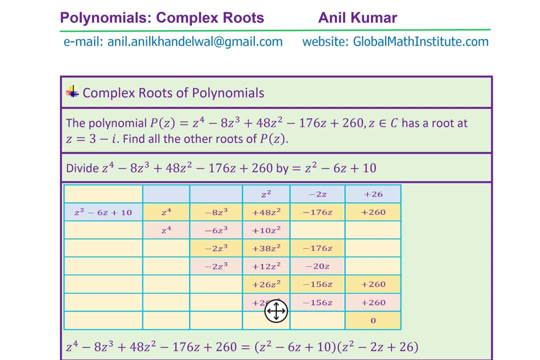 So that's what we are going to do now. So now we are doing long division. So this is the step. We are doing long division. Let me write down long division. So we have z to the power of 4 minus 8z cube plus 48z square minus 176z plus 260.. 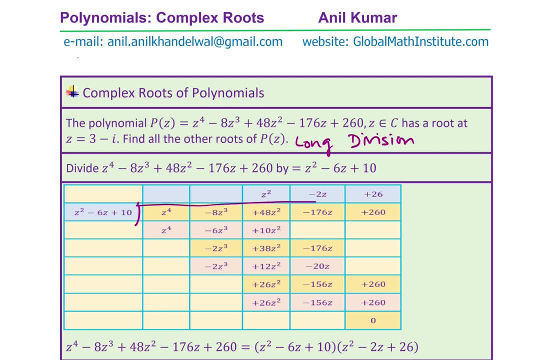 So we are performing this division. now Let me write down the normal symbol for division Right. And we are going to divide this by the factor z square minus 6z plus 10.. Performing this division. now Let me write down the normal symbol for division. 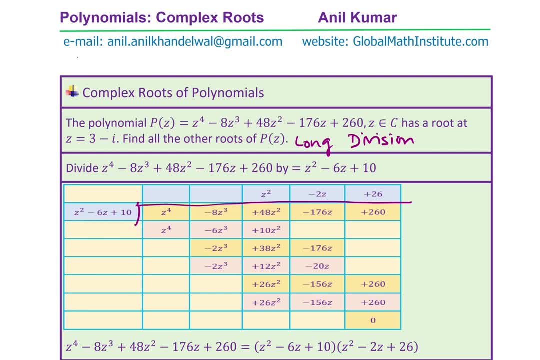 Performing the long division. first, multiplying by z square, z square goes into the quotient and then we have the terms z to the power of 4 minus 6z cube plus 10z square. when we multiply this z square with all the terms right. 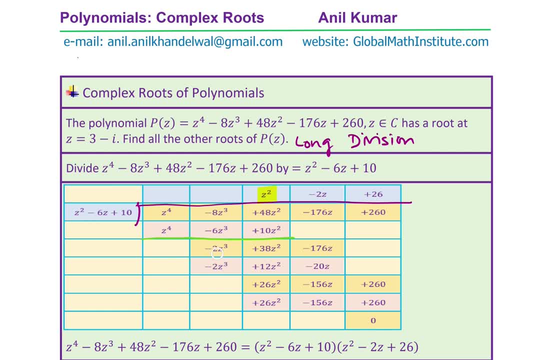 Now you take away. so when you take away you get minus 2z cube plus 38z square minus 176z To get rid of minus 2.. Right Z cube will take the quotient as minus 2z. So we get minus 2z cube here and there are the terms being plus 12z square minus 20z. 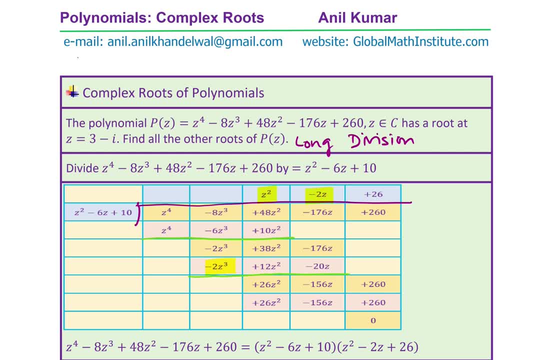 Now take away this. So when you take away, what do you get? You get 26z square minus 156.. Bring down the constant: 260.. And now we need to have 26 on the quotient. So the next term will be plus 28z. 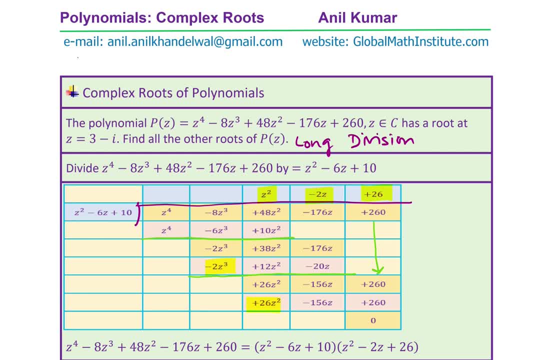 So the next term will be plus 26, which gives you plus 26z square minus 156z to 60 and, as expected, the remainder is 0, right. So that means we have the other factor, which is z square minus 2z plus 26.. 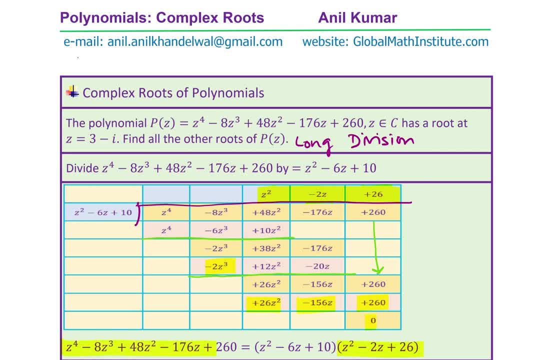 So that is how we could now factor the given polynomial in terms of two quadratic factors, one for which we were already given the complex rules and the other one which we just found To find the other remaining rules. we can actually use the quadratic formula here, and 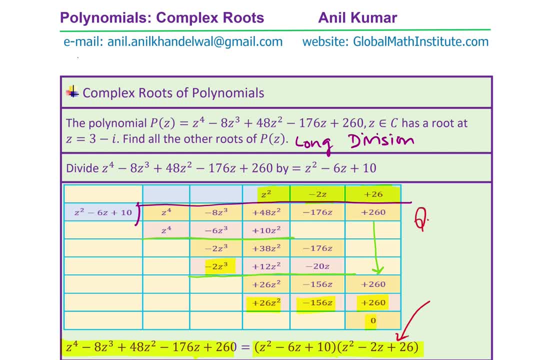 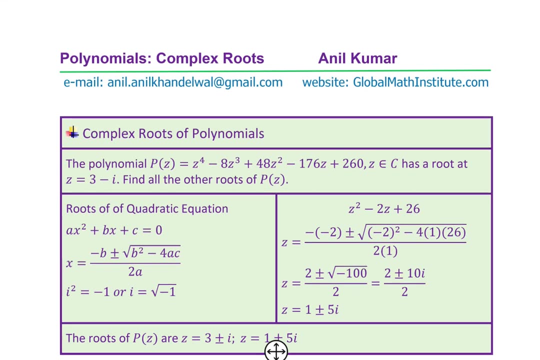 factor this Correct. So now the next step is to use quadratic formula And then factor. So that's what we are going to do now. As a quick reminder, if the equation is of the form ax square plus bx plus c equals to: 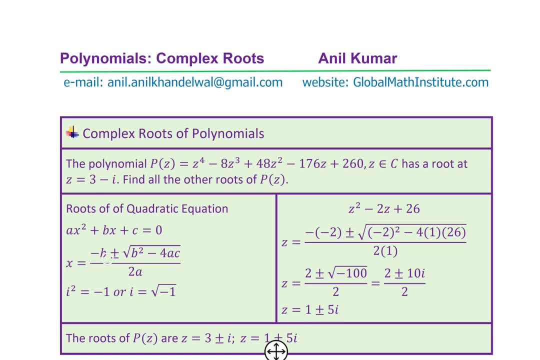 0.. In that case The quadratic formula is: x equals to minus b plus minus square root of b, square minus 4ac over 2a. We are working in the set of complex numbers where i square is minus 1 or i is minus 1. 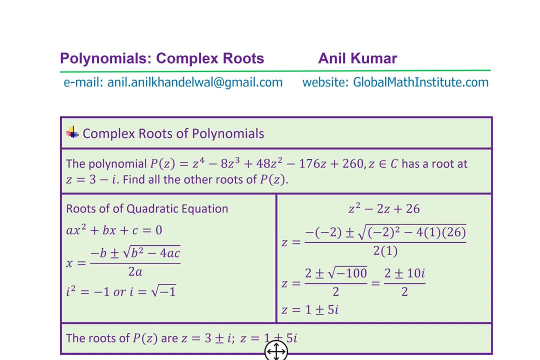 square root Correct. So our equation to work with is z square minus 2z plus 26, where a is 1, b is minus 2 and c is 26.. Substituting the values minus of 2 as b Right.